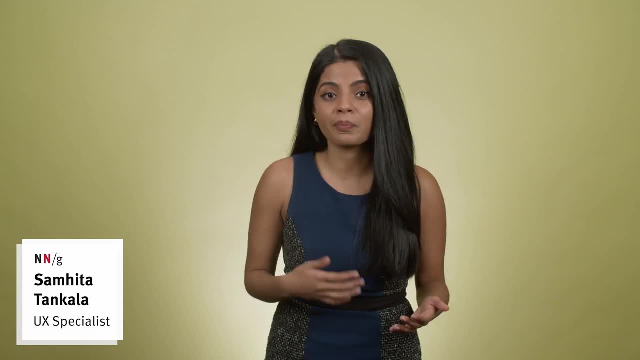 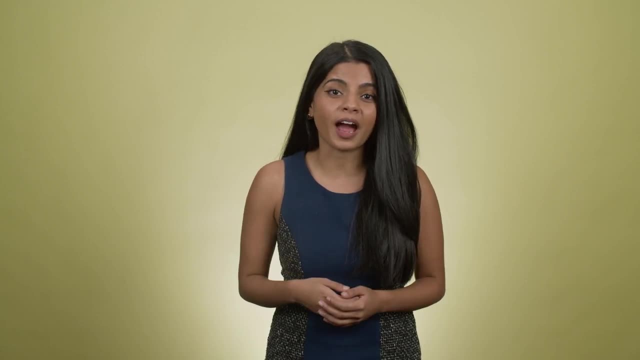 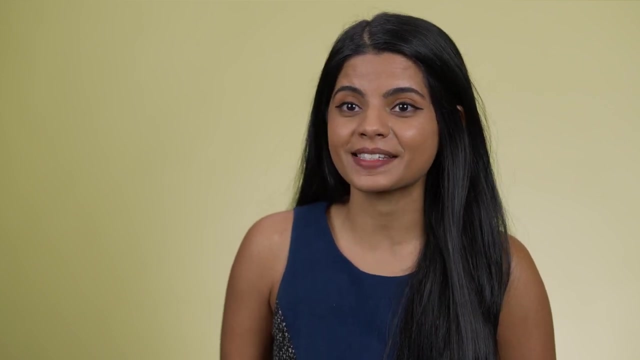 It involves asking participants about their identity, background and who they are today When recruiting participants. these questions are also the first interaction with the study. How can we design good demographic questions during participant recruitment and put participants at ease? First, be mindful of the granularity of your response ranges. 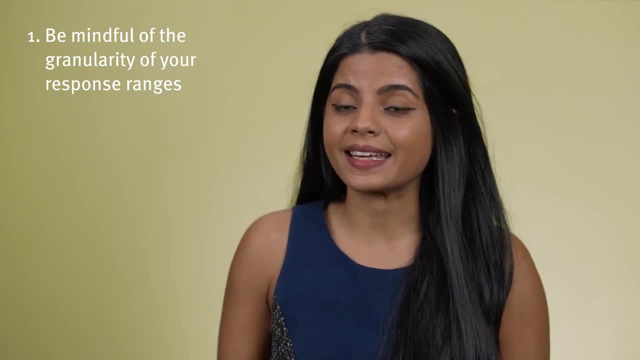 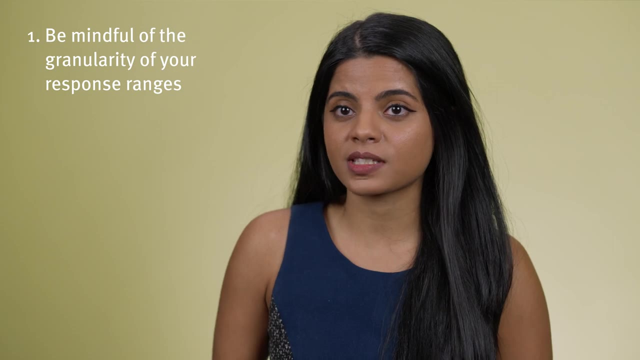 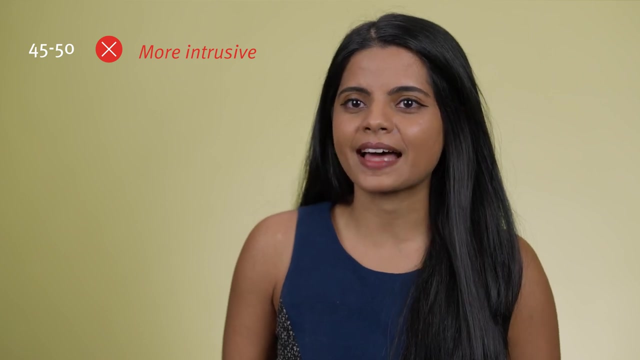 Narrow ranges or questions that require an exact response can be perceived as more intrusive. You want to be mindful of those response ranges. For example, asking someone if they're between 45 and 50 is a lot more intrusive than asking them whether they're between 30 and 50.. 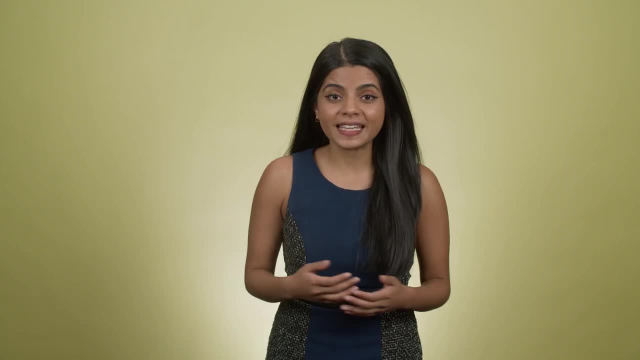 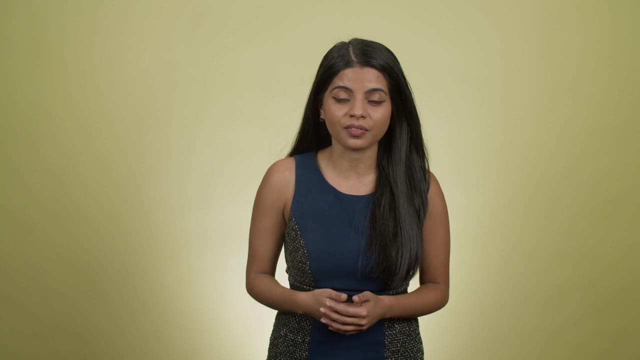 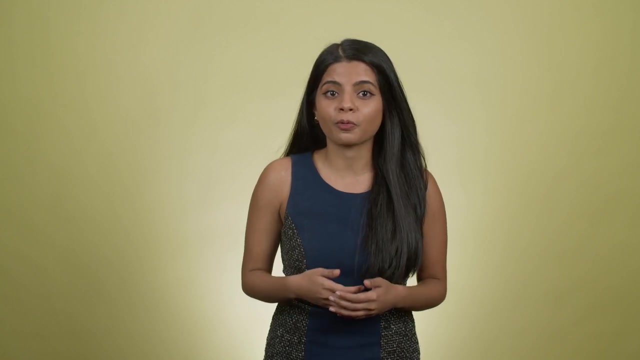 But this doesn't only apply with age demographics. When it comes to income, asking them if they make between $70,000 and $80,000 will be perceived as more sensitive than asking them if their income is over $50,000.. If you have a good reason for using narrow ranges, provide participants with an explanation why you need this information. 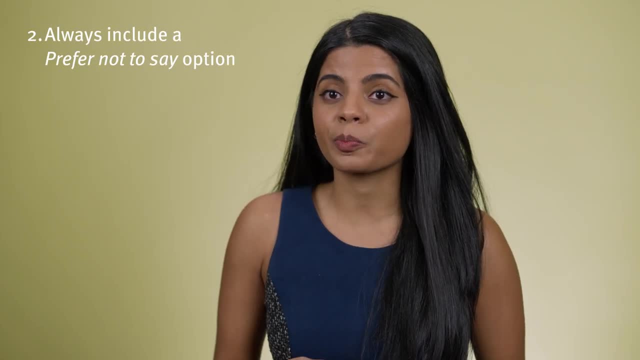 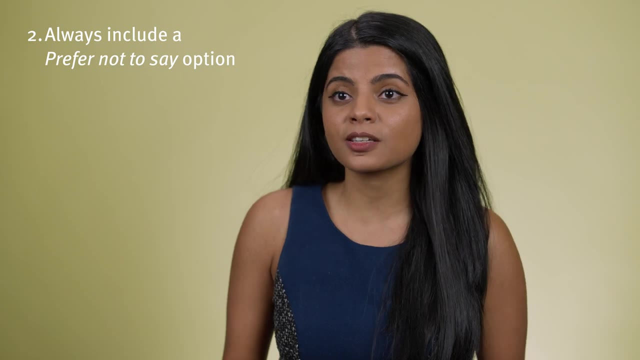 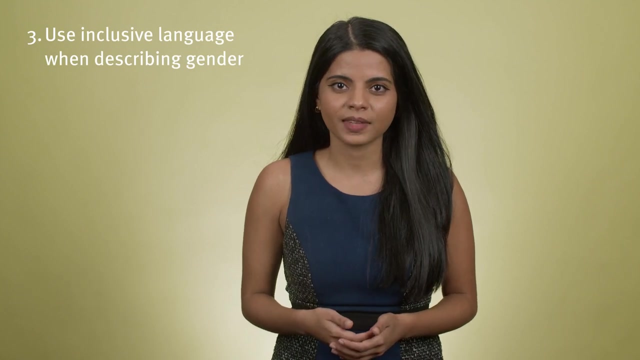 Second, always include a prefer-not-to-say option. This option provides participants a way out and may encourage participants to continue the survey and not feel trapped. Third, use inclusive language when describing gender. Always give participants the option to describe what they currently identify as. 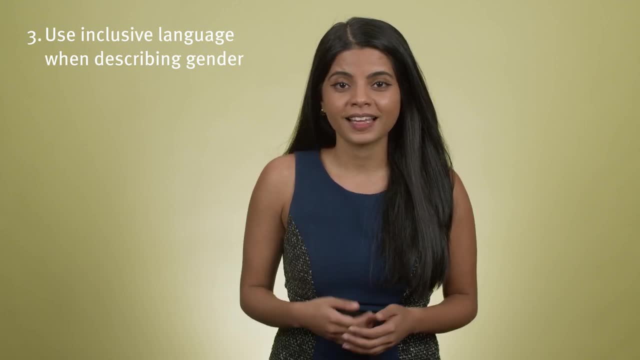 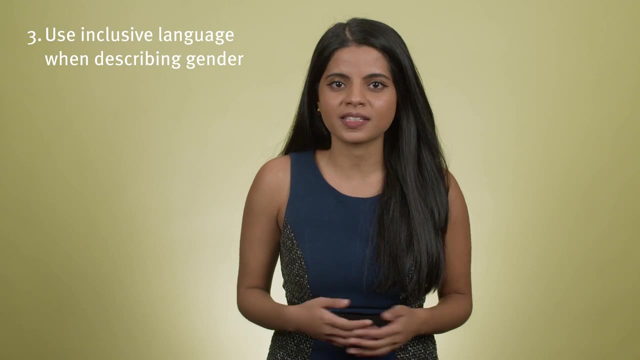 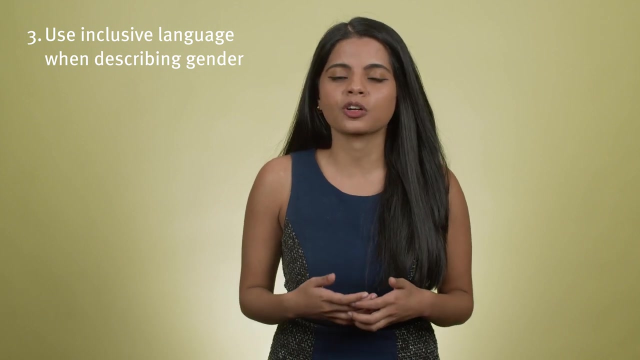 Gender can change over time. Language around gender is also constantly evolving. For example, 10 years ago, a question may have been listed male and female as the only gender options, But now you should think about including terms like non-binary transgender, to put everybody at ease. 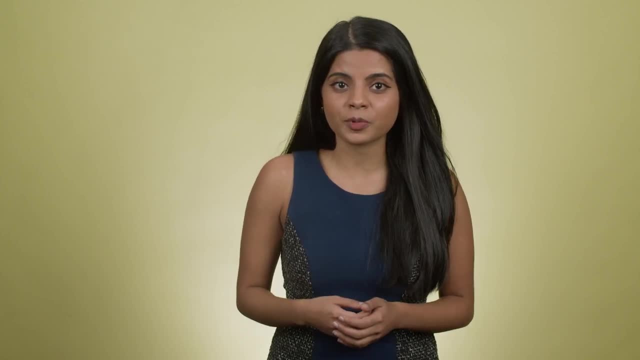 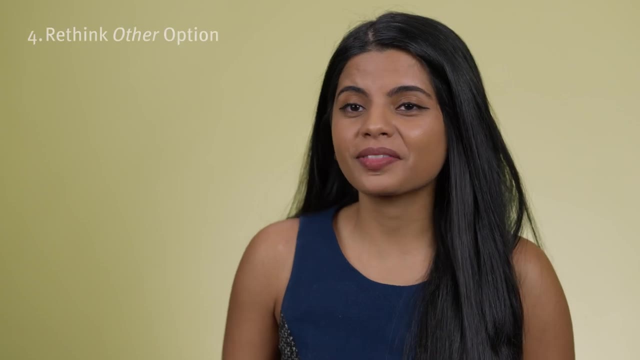 You should also include a prefer-not-to-say option so participants can opt out of the question if they aren't comfortable selecting a gender. Fourth: rethink the other option. It's always good to include an option where participants have the choice to explain.